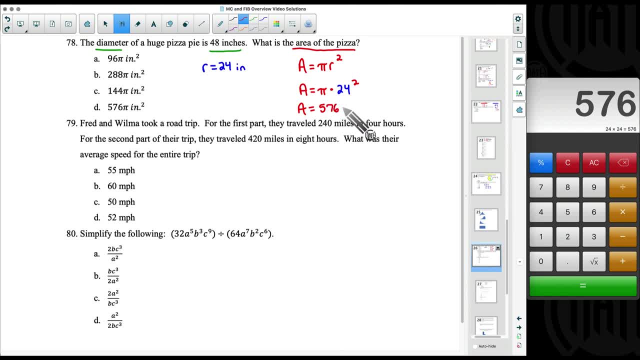 But I'm going to go ahead and write the 576 in front. Then we can put the pi after it. That means the same thing. because we are multiplying here, Our answer is going to be D, Number 79.. Fred and Wilma took a road trip. For the first part, they traveled 240 miles in four hours. For the second, 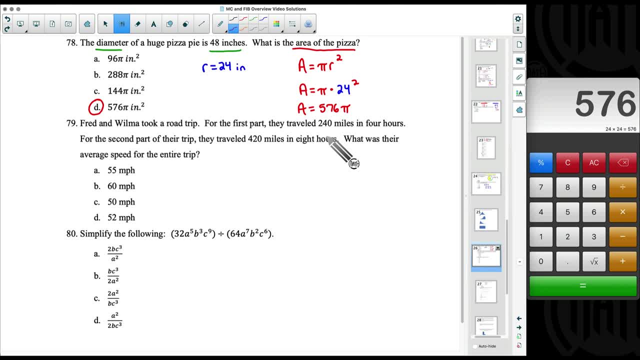 trip. they traveled 420 miles in eight hours. What was their average speed for the entire trip? What you don't want to do, We're trying to find the average speed for the entire trip. You don't want to find the average speed here and you do not want to find the average speed here. 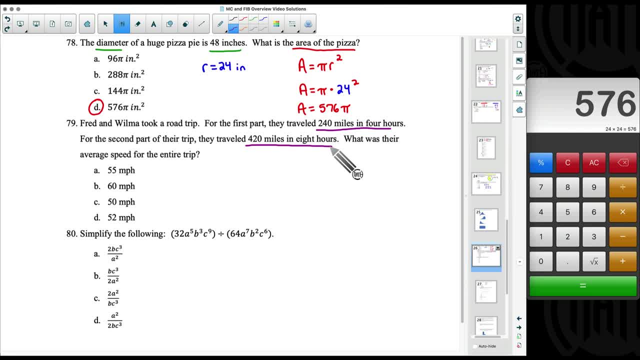 and then add those up and divide by two. That does not always work, And the reason why that's not going to work here is because we have two different time intervals. The first part of their trip they drove for less time than they did on the other side, So they drove for less time than they did on the 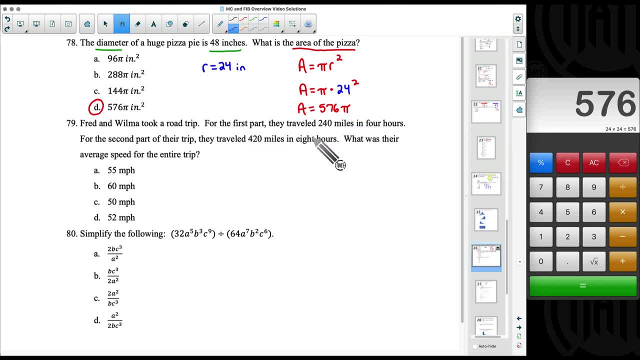 second part of their trip. The way to find the average speed for the entire trip, Take the total distance and that total distance is going to be 240 plus 420.. So 240 plus 420. Their total distance is 660 miles. Take your total distance and divide by the total time- Four hours and eight hours We. 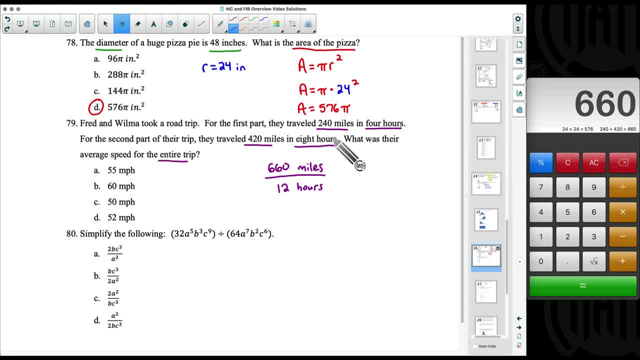 get an average speed of 55.. And something else I want you to notice: here too, We do see MPH. Well, technically that is miles per hour. That's exactly where that's coming from When I wrote the miles over the hours Now, you would not get that answer had you found the average speed for the. 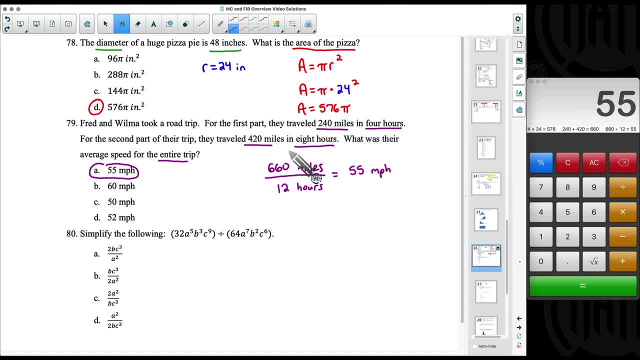 first part, Then the average speed for the second part, And then if you try to do something with those, That is not how you find the average speed for the entire trip. Now number 80. We're doing some algebra, We're trying to divide here. Now, when you're dividing, you can think of this as a 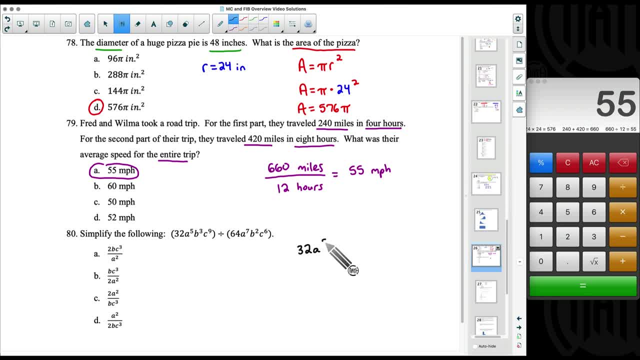 fraction. So I'm just going to change the way this looks, But it's going to mean the same thing. So this first part, 32 a to the 5th, b cubed c to the 9th, We can put all of that over Because 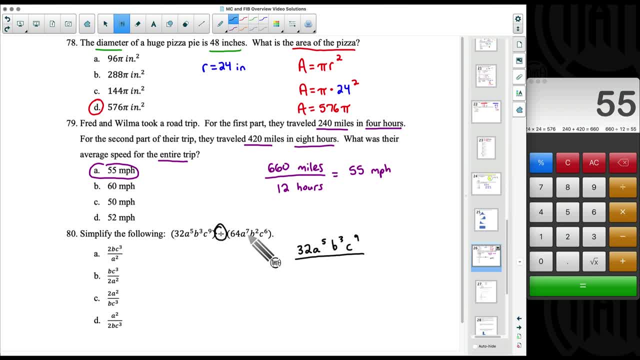 it's going to be a fraction, So it's all of this stuff over this stuff right here at the bottom. So I'm going to write that Now we don't have any addition or subtraction, Like we don't have a plus or a minus up here And we don't have that down here either. And if we did, it would make this: 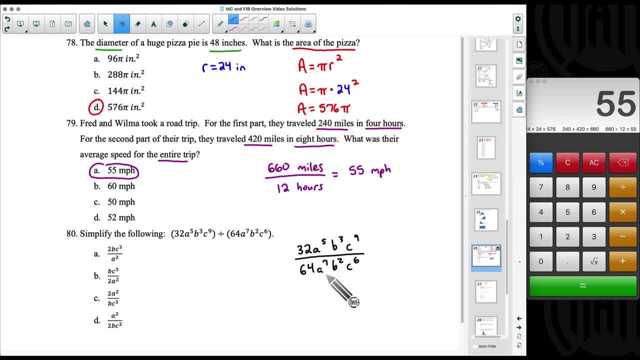 problem much more complicated Or maybe even impossible to simplify- You don't have to worry about that for the t's- But what we can do, Since we don't have any of that addition or subtraction going on, Let's focus on our numbers first. 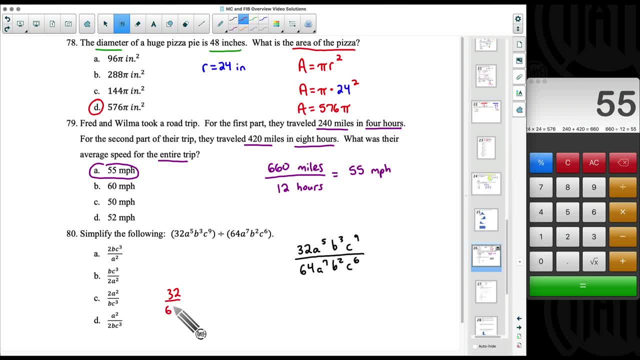 Let's take the 32 over 64.. And you need to simplify that fraction. You can divide that. You'll get 0.5.. 32 divided by 64 is 0.5.. That's the same thing as one half. But notice if I simplify. 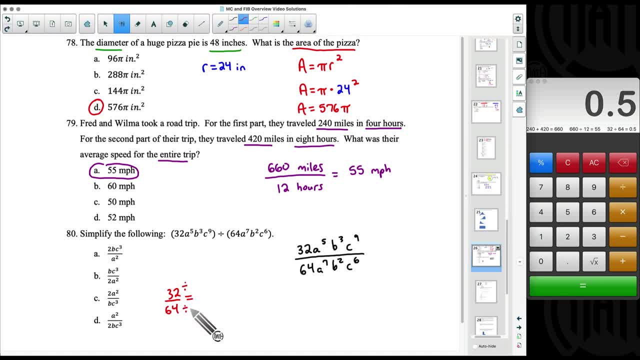 here Now. you can divide by a whole bunch of different things. You can divide by 2.. You can divide by 4.. You can divide by 8.. You can divide by 16.. Heck, you can even divide both of these by 32.. 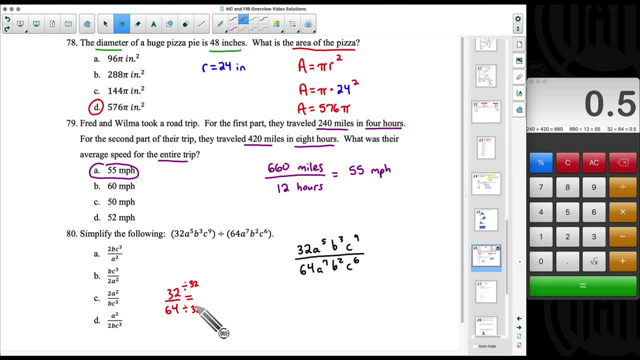 So simplifying. you have a lot of options, But 32 is the greatest common factor, That's the biggest number that we can divide both of these by, And 32 divided by 32 is 1.. 64 divided by 32 is 2.. So notice, we do get one half. So this: 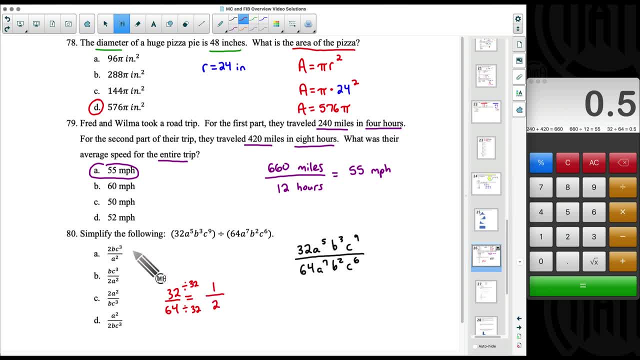 means we have a 1 at the top and a 2 at the bottom. Automatically we can eliminate A and we can eliminate C, Because the 2 is at the top. We want the 2 at the bottom, And you may wonder well. 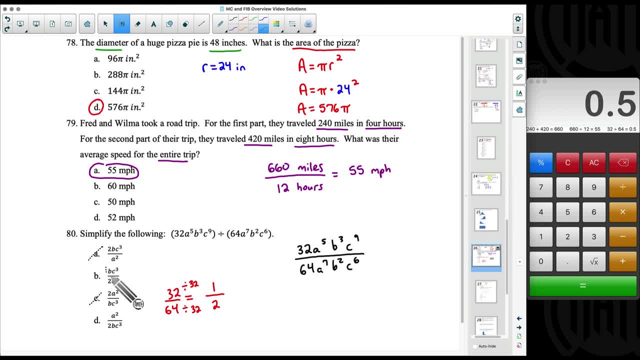 what about this 1?? I mean, I can stick an understood 1 here in front of that BC cubed. I can stick an understood 1 there in front of the A squared. We don't need it there. That's why you don't see it. 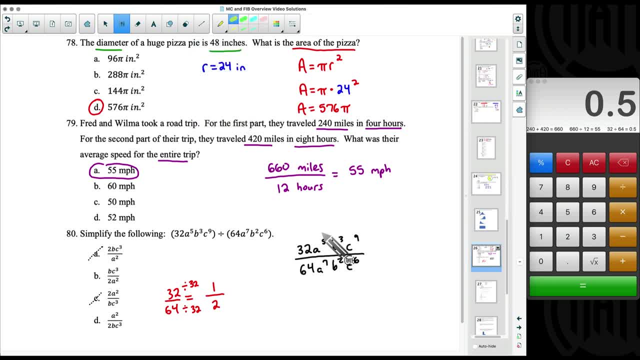 But there is an understood 1.. Now let's move on to our variables. Wherever you have more variables at, so to speak, A to the 5th over A to the 7th, We have more A's at the bottom. How many more do we? 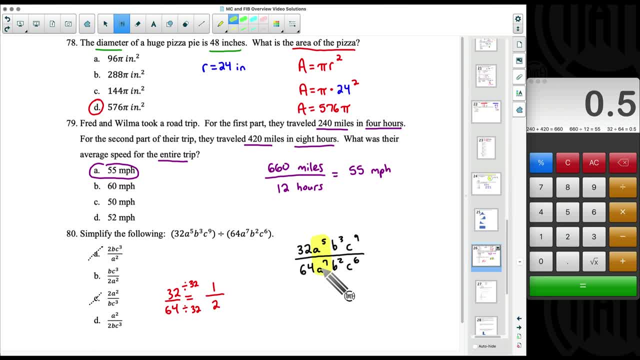 have Two. The rule here is you subtract exponents And we're dealing with just the A's. Don't worry about the B's or the C's. But again we have more A's at the bottom, So we want our A to be at the. 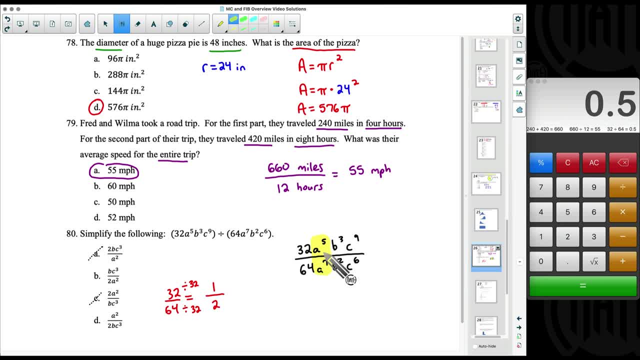 bottom And we have two more A's at the bottom than we do at the top. There's our A squared Notice: A squared is in the wrong spot for D. We don't want it at the top. We had more A's at the. 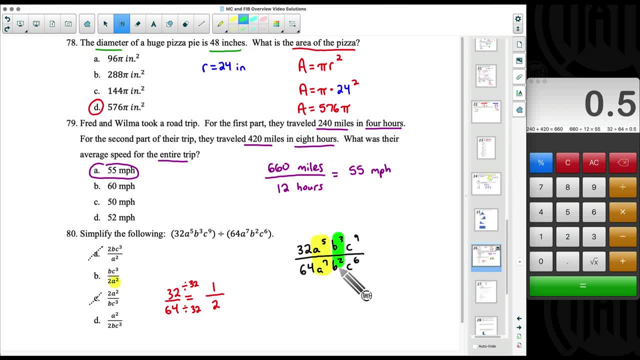 bottom. And since we're on a roll here, let's go ahead and look at the B's. We have more B's at the top. How many more B's do we have at the top? We have one extra B. 3 minus 2 gives us 1.. Well, that right, there is a B to the understood first power. If you don't see, 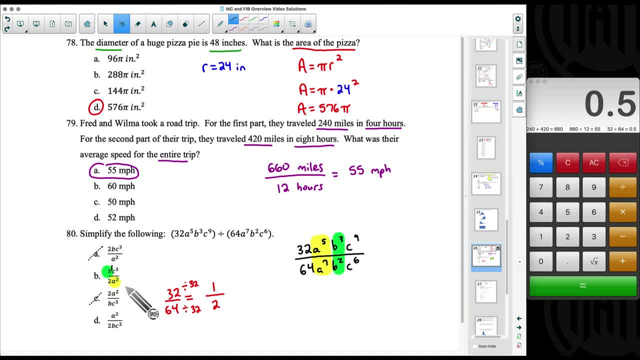 an exponent with a variable, it's automatically raised to the first power Understood 1 there again. And then, last but not least, let's look at our letter C. Where do we have more C's at? We have more C's at the top C to the 9th. 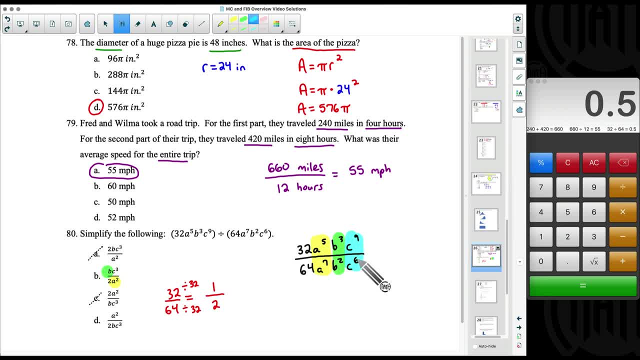 How many more C's do we have? 9 minus 6 gives us 3.. So we have C cubed left at the top. Our answer is going to be B. Now let's jump into the workbook for some additional tips. So here's number. 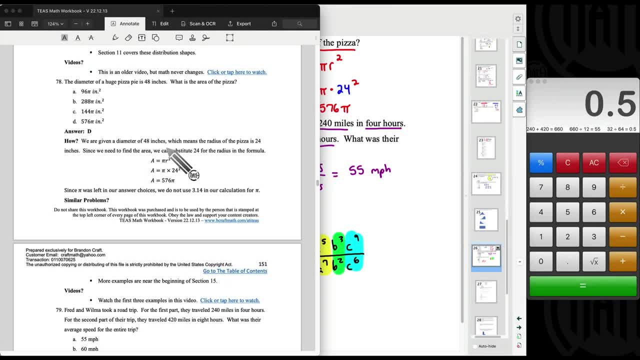 78. We did say our answer was D, We're given the diameter. You got to find the radius in order to find the area of a circle. Apple pies are 2.. So don't forget that when it comes to circles, Even 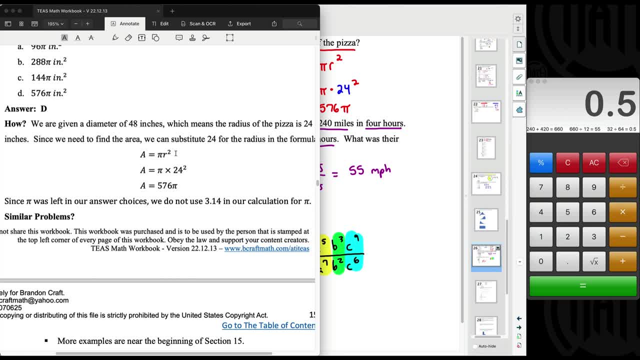 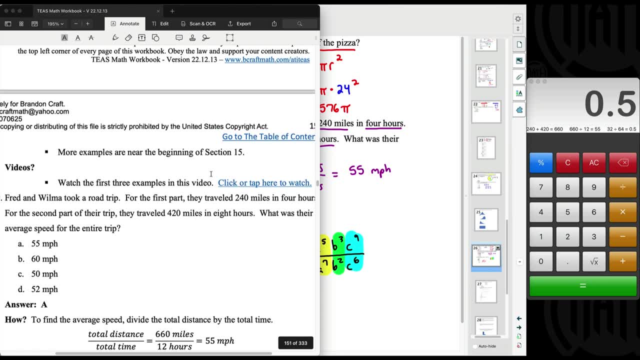 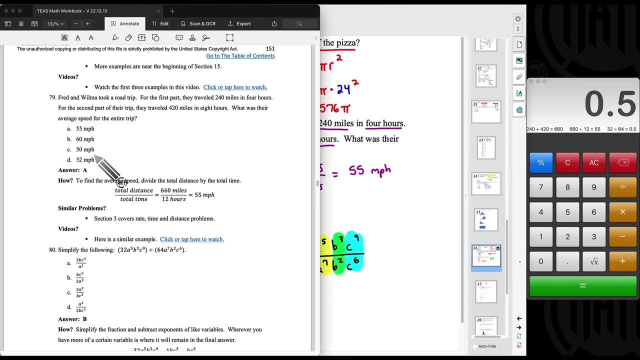 though we didn't deal with circumference. Apple pie is delicious. Apple pies are 2. We definitely use the apple pies there, Section 15.. More circle problems. First, three examples in this video. Watch that for additional examples 79. I did mention. take the total distance and divide by the total time. That's how we got 55. 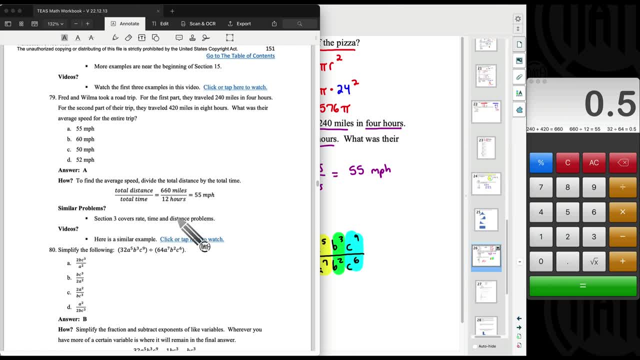 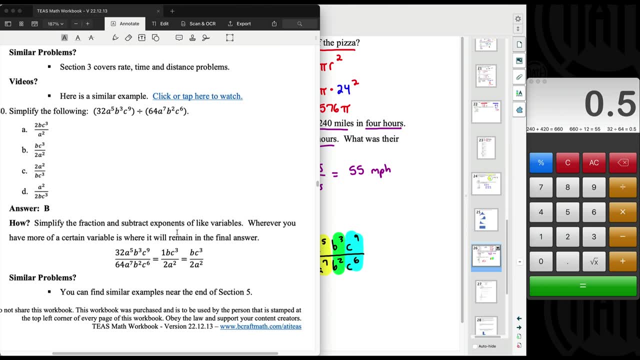 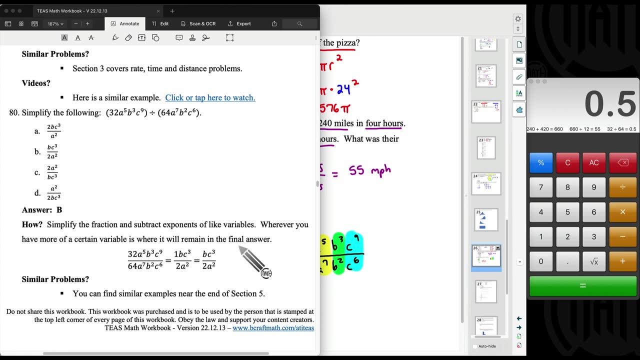 miles per hour. Section 3.. Rate, time and distance problems- Additional video there. Then number 80.. We did turn this into a fraction And I mentioned wherever you have more of a certain variable is where it will remain. in the answer I was asking you: where did we have more A's, Where did we have more B's, Where did 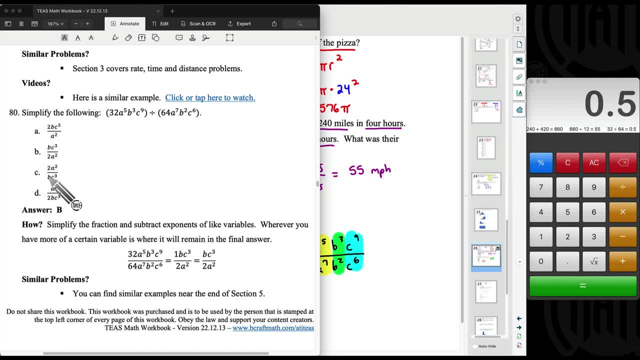 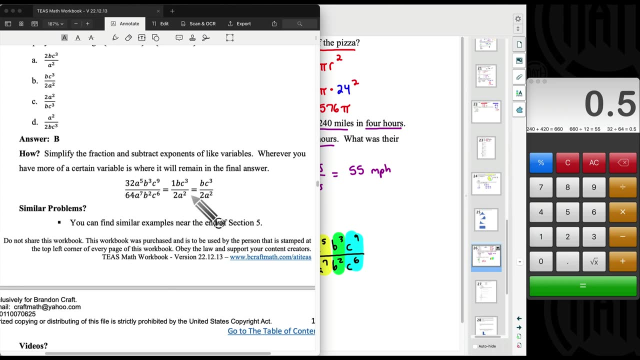 we have more C's And we even eliminated our answer choices based on that. And then just bear in mind being able to simplify fractions with just numbers like the 32 over 64.. Look at the end of section 5 for additional examples there. Section 5 mainly deals with the equations, but I did include